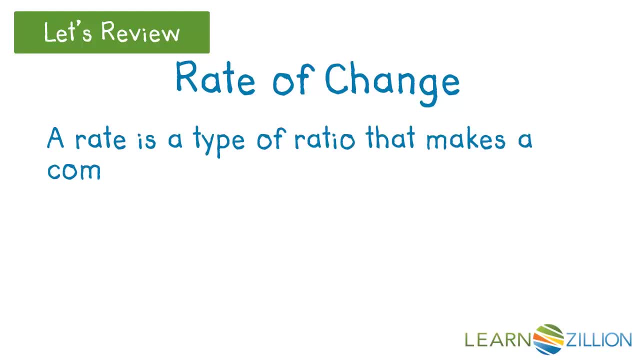 You probably remember that a rate is a type of ratio that makes a comparison between two measurements with different units. The two measurements give us the numbers to calculate the change in output per change in input. That's our rate of change. Also, don't forget that slope has direction. 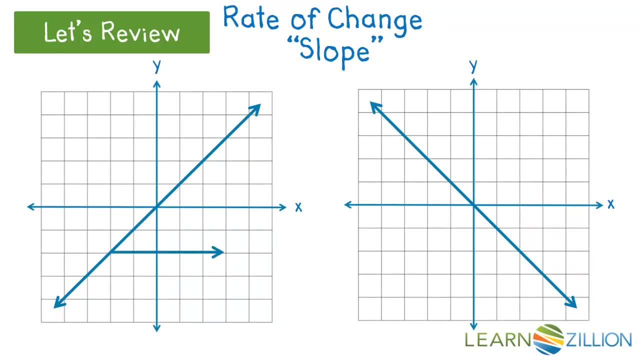 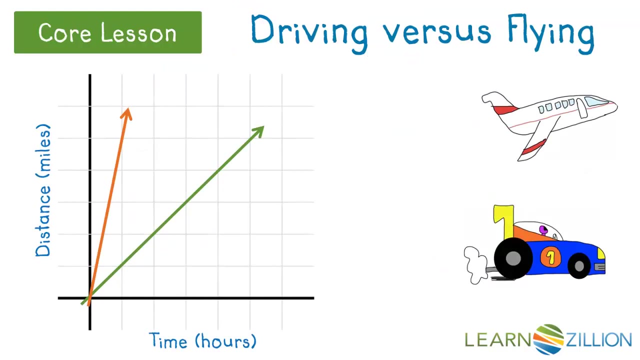 Direction tells you up or down, positive or negative. We will add a number to direction in this lesson to tell us the degree a linear relationship is going up or down. This graph shows how far a car and a plane have traveled As time increases. 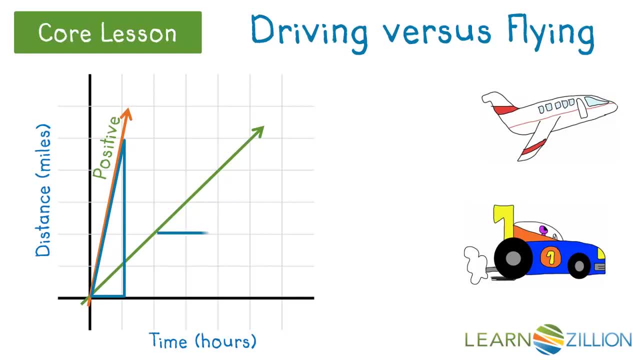 the distance increases for both the car and the plane. So they are both positive, But they are different, right? Can you tell which one is the plane? The plane increases distance a lot faster than the car, So the orange line represents the plane. 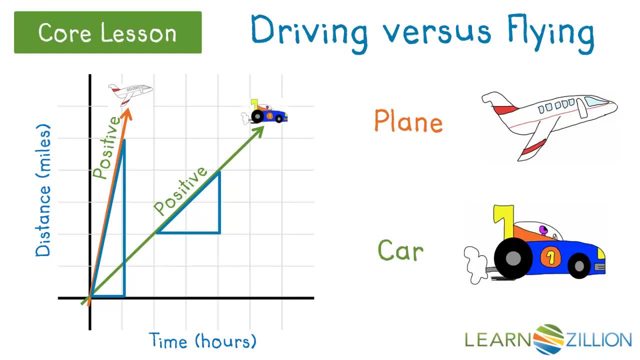 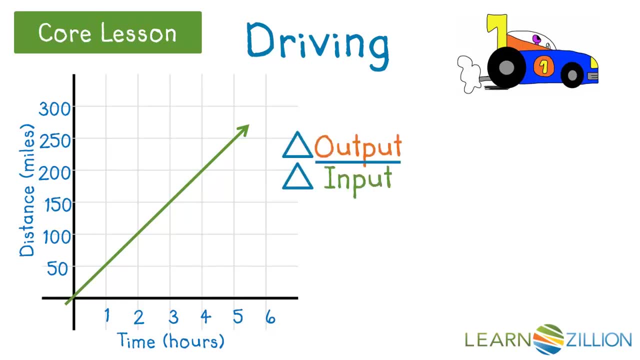 and the green line represents traveling by car. Let's look a little closer at traveling by car. Rate of change is a ratio of change in output to change in input. There's a triangle in front of these terms to represent change in. Sometimes we call it rise over run. 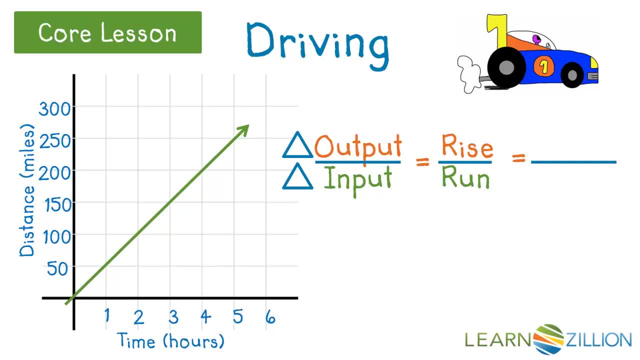 How much does the line rise up or down? to how much does it run left or right? So let's start at the origin of the graph and look at a change in one hour. I included a plus sign, so you know we're increasing one hour. 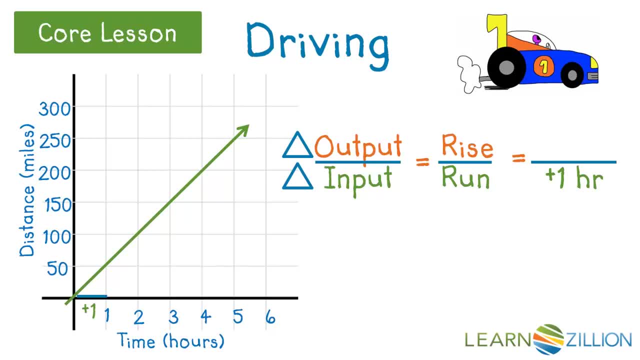 I recommend you always do the same. So as we increase one hour, what happens to the output- Positive 50 miles? A change in output of positive 50 miles to a change in input of plus one hour is 50 miles per hour our rate of change. 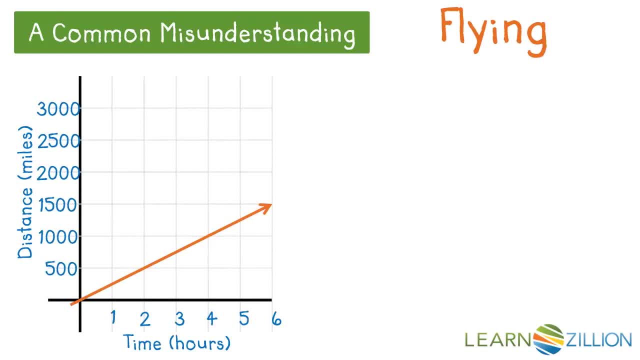 A common misunderstanding is looking at how steep the line is and thinking this is a smaller slope than the graph. before Using the scale is critical to determine the change in output. Here the change in output is 750 miles for a change in positive 30 miles. 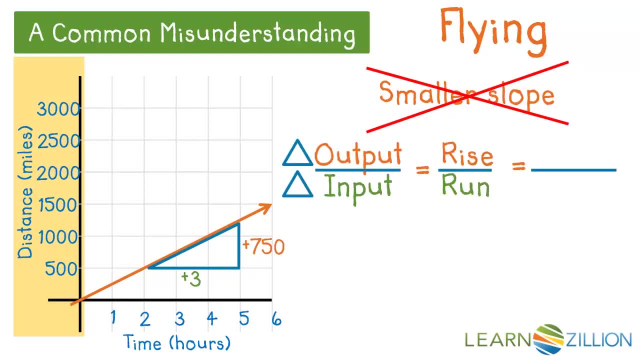 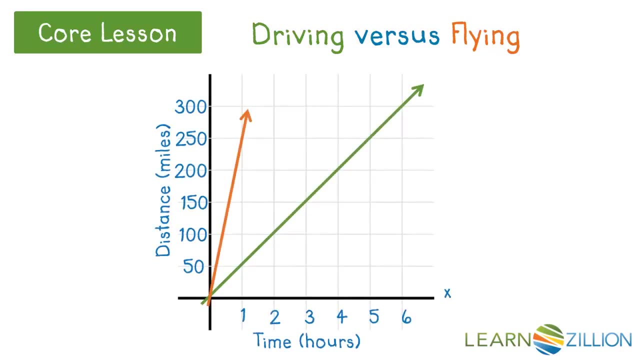 When we calculate the slope, 750 miles over three hours gives us a rate of change of positive 250 miles per hour, much faster than a car. When both lines are plotted on the same graph, it's much easier to compare the slopes and see that flying is a lot faster.